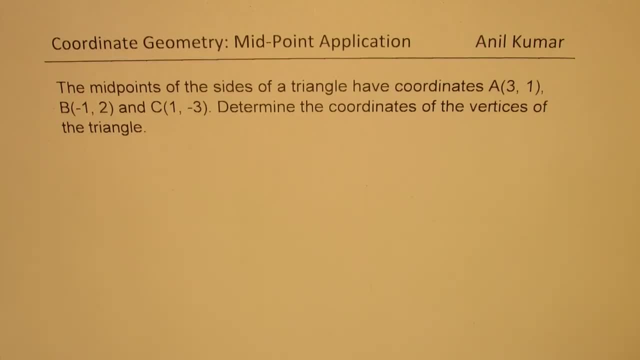 I am Anil Kumar. Welcome to my series on Coordinate Geometry. We have a wonderful test question here, which is an application of midpoint. You can always pause the video, copy the question answer and then look into my suggestions. The question here is: the midpoints of the sides of a triangle have coordinates a- 3, 1, b minus 1, 2 and c- 1, minus 3.. 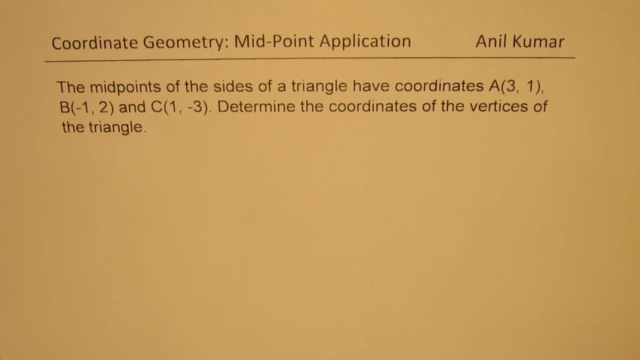 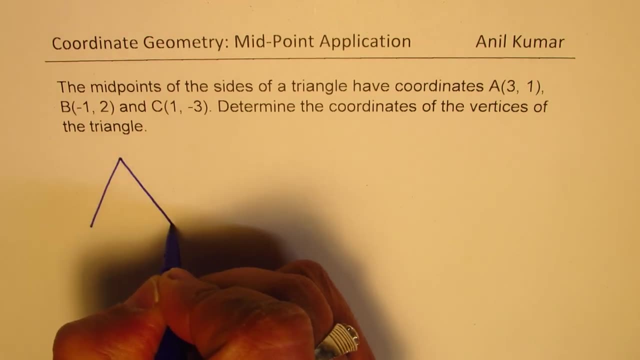 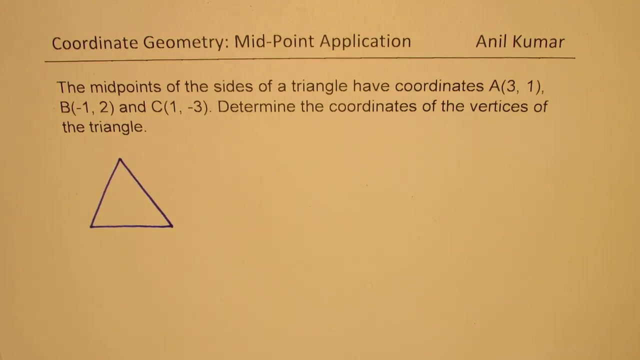 Determine the coordinates of the vertices of the triangle. So let's sketch the triangle first and then we'll work on this. Let us say that's the triangle whose midpoints are given to us. So midpoints, let's say a is given to us as 3, 1.. b is minus 1, 2.. 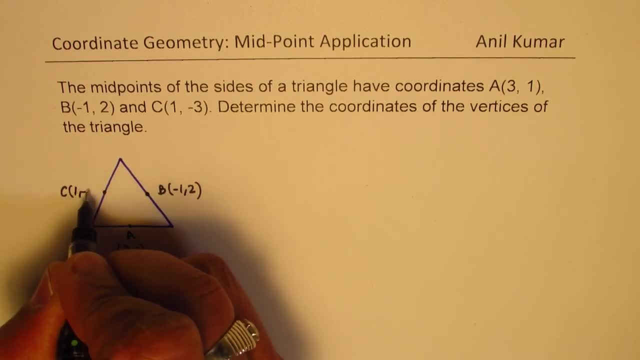 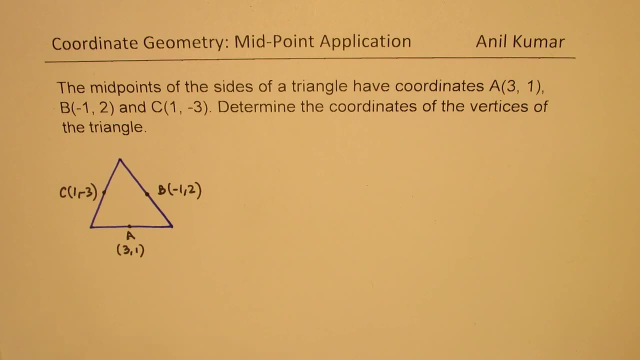 And c is 1, minus 3.. We need to find the vertices. that is, d, e and f. Okay, so let this be d. We can call this as x 1, y 1, e, x 2, y 2 and f x 3, y 3.. 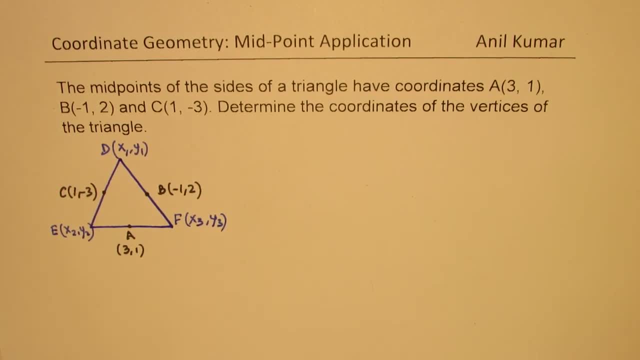 So that is what we need to find. Well, in general, we have the midpoint formula. Let me write down the midpoint formula here, Which basically is that the average of the x values and the y values. we can always say like this: 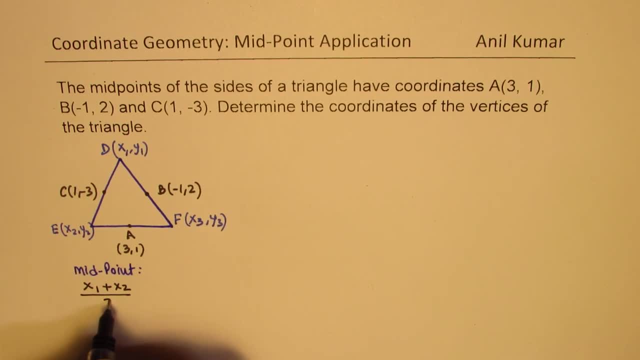 x 1 plus x 2 divided by 2 is equal to what, So x 1 plus x 2 divided by 2 will be 1, in this case correct, And y 1 plus y 2 divided by 2.. 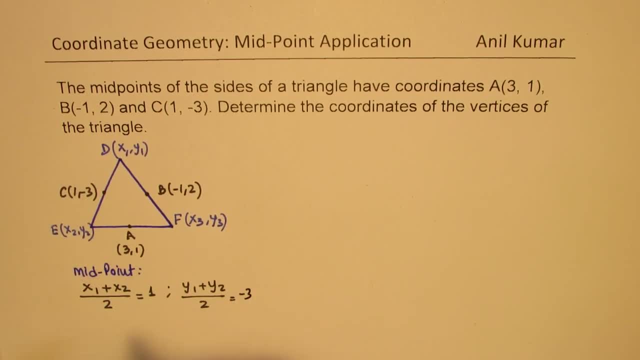 Is going to be the y value of c, which is minus 3.. So if I cross multiply, I get: x 1 plus x 2 equals to 2 times 1.. And y 1 plus y 2 as 2 times minus 3, which is minus 6, correct. 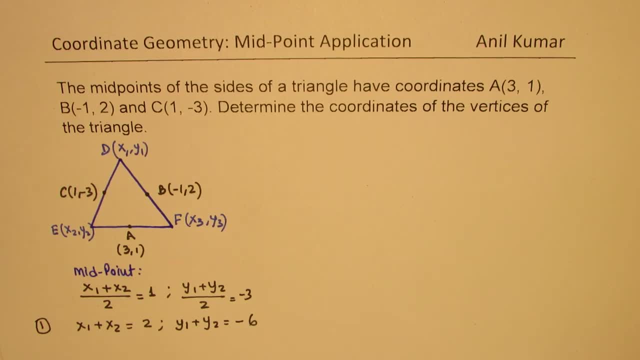 So I get one equation relating x 1, x 2 and y 1, y 2.. Well, I could do this for all the three points correct, So next time Let's take these two. 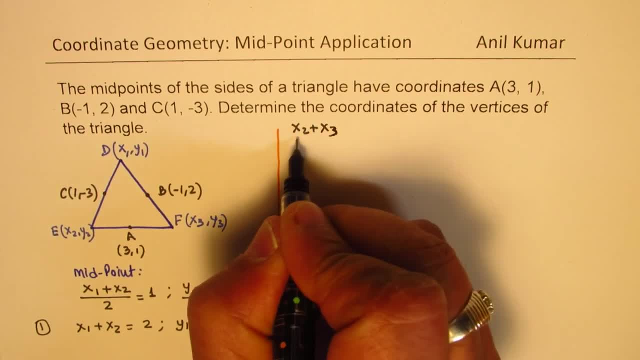 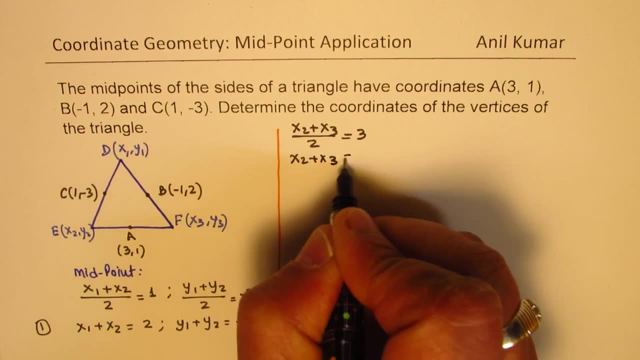 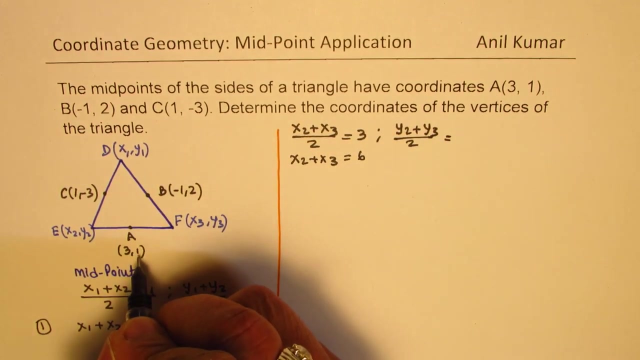 So we say x 2 plus x 3 divided by 2 is equal to 3.. So that means x 2 plus x 3 is 6.. And we have: y 2 plus y 3, divided by 2 is 1.. 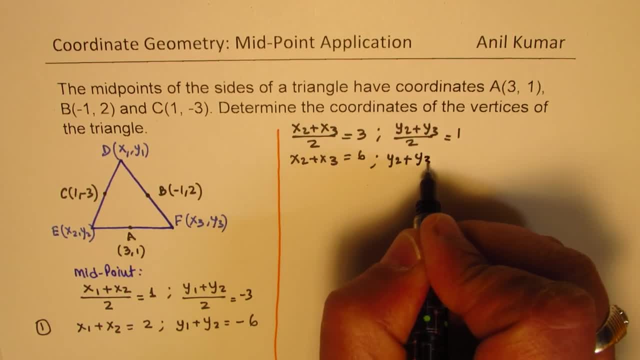 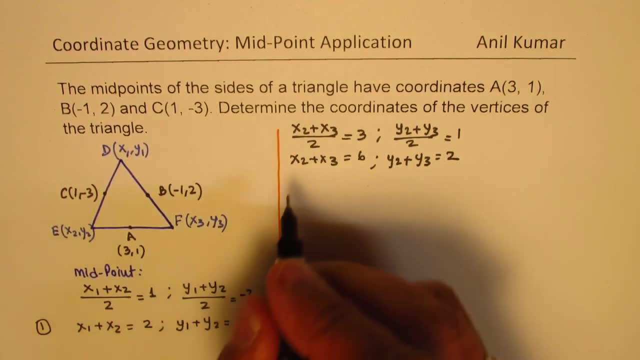 So we have y 2 plus y 3 equals to 2, right. And uh, So we have y 2 plus y 3 equals to 2, right. Similarly, x 1 and x 3.. 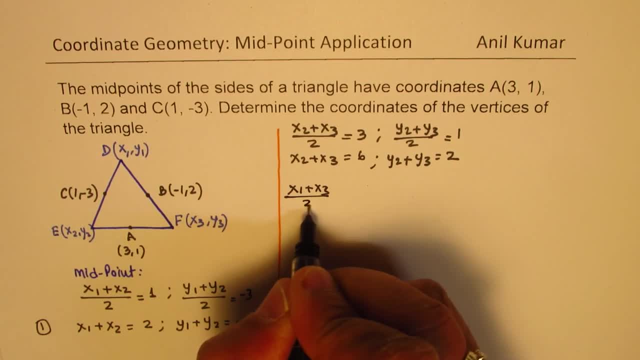 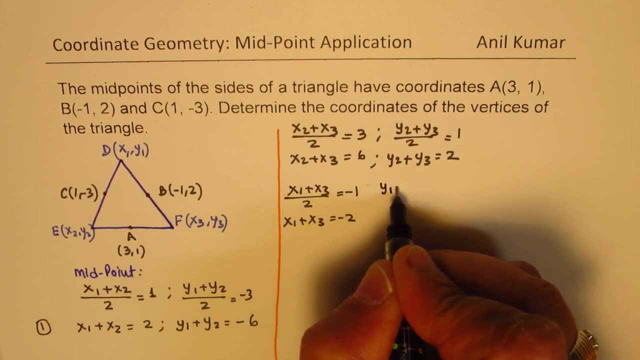 So we have: x 1 plus x 3 divided by 2 is minus 1.. x 1 plus x 3 is minus 2.. And y 1 plus y 3 divided by 2 is 2.. 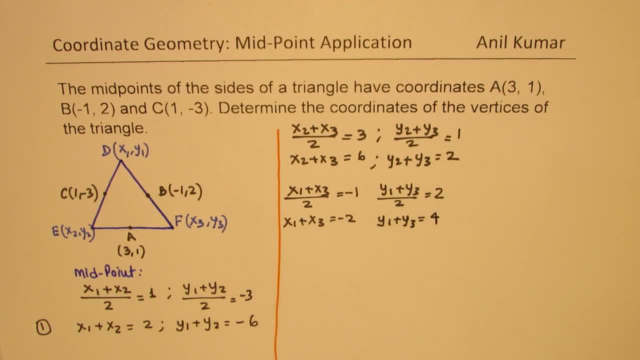 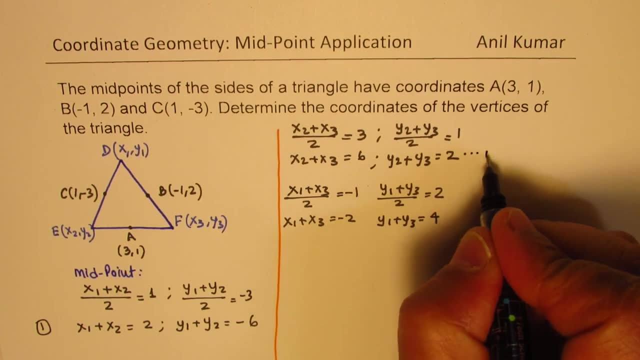 y 1 plus y 3 is 2 times 2,, which is 4.. So, as you can see, we get these three equations which relate x 1, x 2, y 1.. 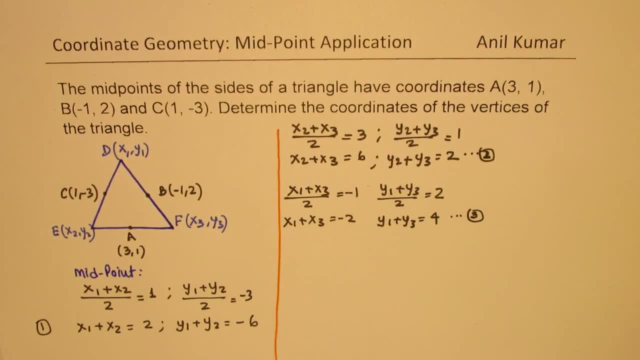 y, 2, right, All these. Now what happens when I add equation 1,, 2, and 3?? That is interesting See. what we have here is something like this. We are writing: x 1 plus x 2 equals to 2, right. 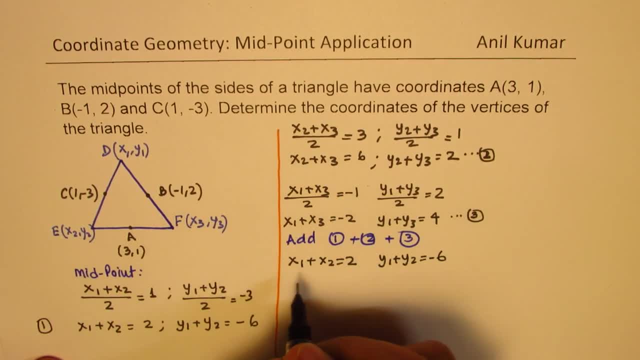 y 1 plus y 2 equals to minus 6.. Then we got x 2 plus x 3 equals to 6.. y 2 plus x 3 equals to 2.. y 2 plus x 3 plus y 3 equals to 2.. 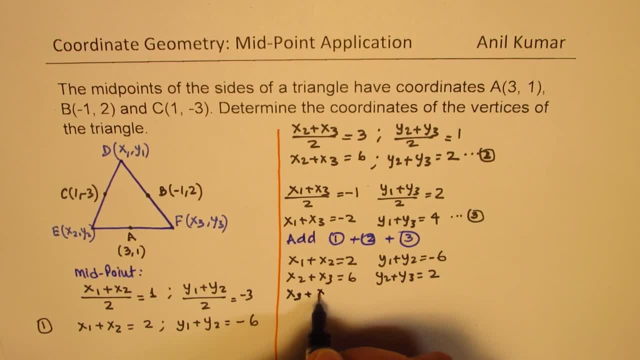 And we get x 3 plus x 1 minus 2. And y 1 plus y 3 as equals to 4.. Now if I add them, then we get twice x 1,, twice x 2, and twice x 3.. 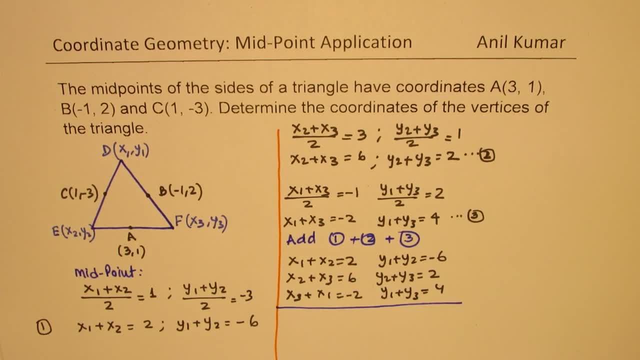 I rewrote this just to show you clearly that we get 2 times all these values right. So we get 2 times x 1 plus x 2 plus x 3.. As equal, to add them all, which is 6.. 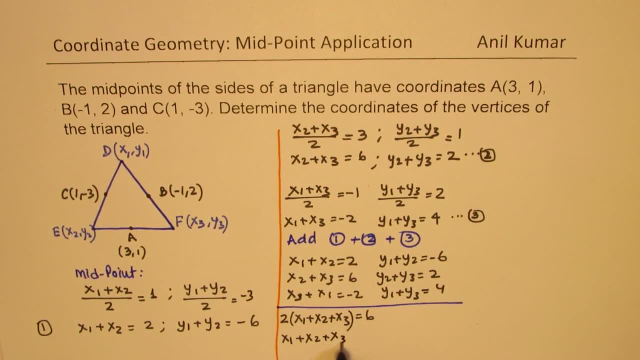 Or x 1 plus x, 2 plus x 3 is half of 6,, which is 3.. Here we get y 1 plus y, 2 plus y, 3. 2 times right. 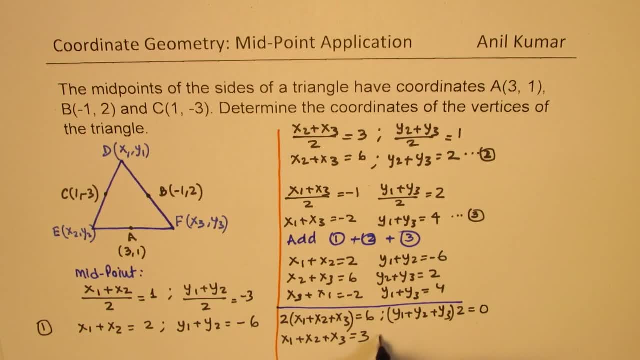 Because when you add it is twice And that is 0. And so we get y 1 plus y 2 plus y 3 equals to 0. So 0 divided by So that should help you to get your answers right. 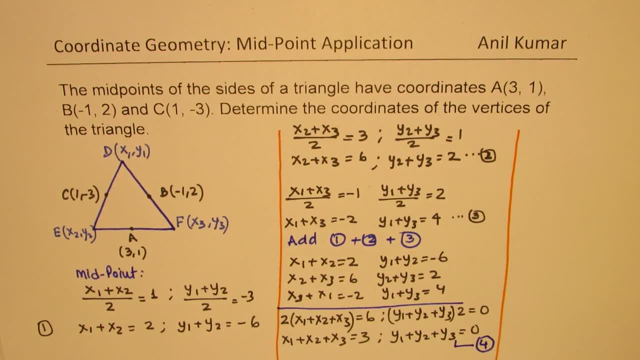 So this is kind of a very critical equation which gives us all the answers. So we can say that if I want what is x 1, from 3,, I have to take out sum of x 2 and x 3, right. 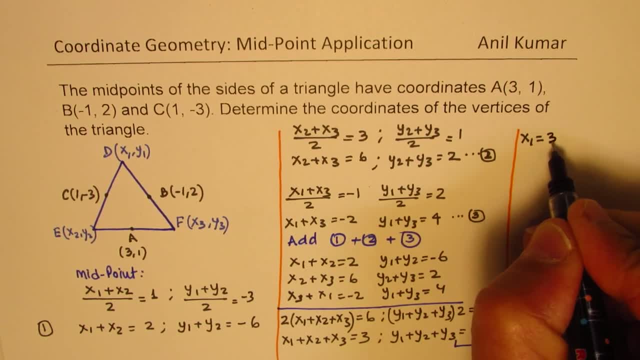 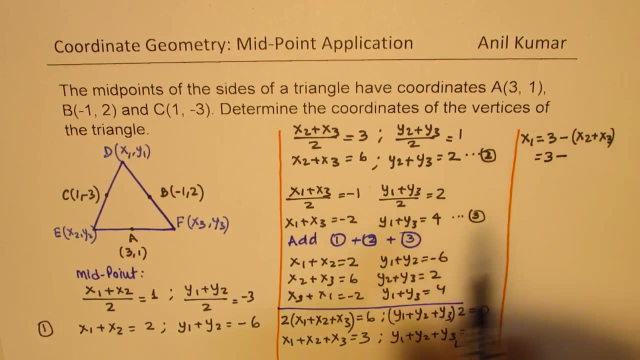 So we can say: x 1 is equals to 3 minus x 2 plus x 3, clear. So which is basically 3 minus? What is x 2 plus x 3?? It is 6.. 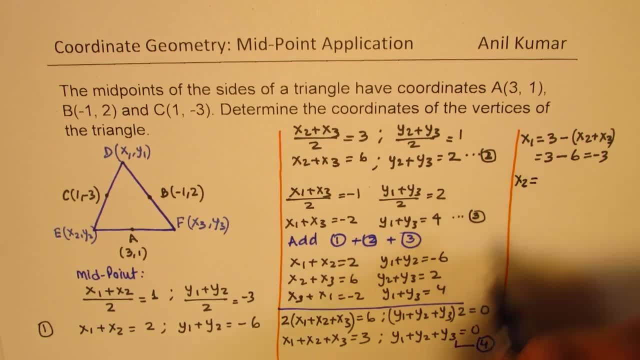 So that is minus 3.. Similarly, I can say: what is x 2?? x 2 will be 3 minus x 1 and x 3, right, So which is minus 2?? So when I do minus 2, I get 5.. 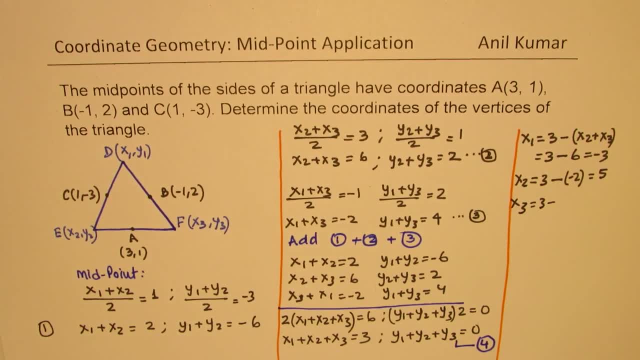 And x 3 will be 3 minus x 1 and x 2 sum, which is 2.. So we get 1, right? So we get one set of x values Now. similarly, y 1 will be 0 minus the sum of y 2 and y 3,, which is: 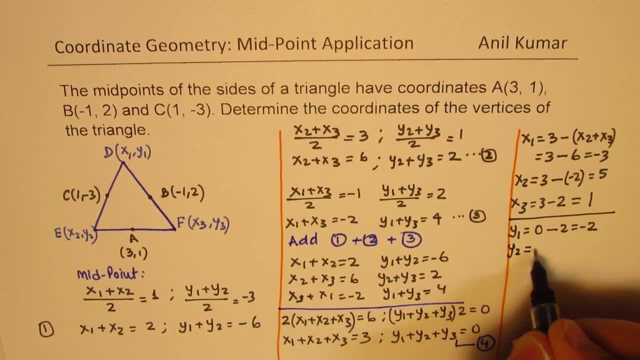 So we get minus 2.. So we get minus 2.. y 2 will be 0 minus sum of y 1 and y 3,, which is 4.. So we get minus 4.. And y 3 is 0 minus sum of y 1, y 2,, which is minus 6.. 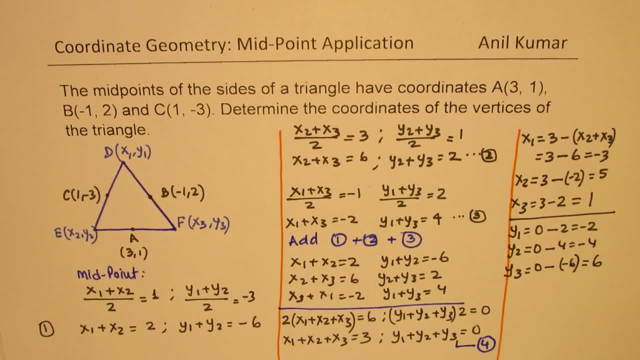 So we get plus 6. Do you see that part? So now we can easily write down our coordinates: d is x, 1. d is x: 1. y, 1. So it is minus 3, minus 2.. 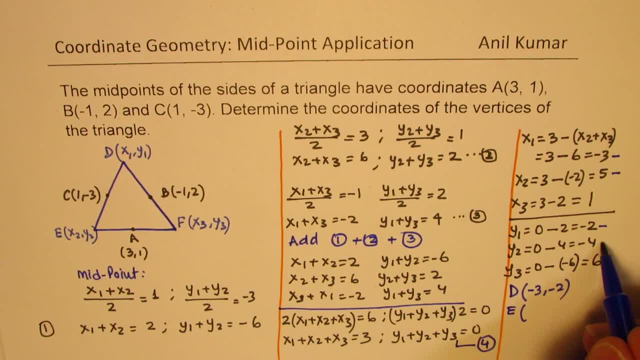 e is x, 2 and y 2.. So it is 5 and minus 4.. And f, which is 1 and 6.. Right, So that is how we get all the points. Does it make sense to you? 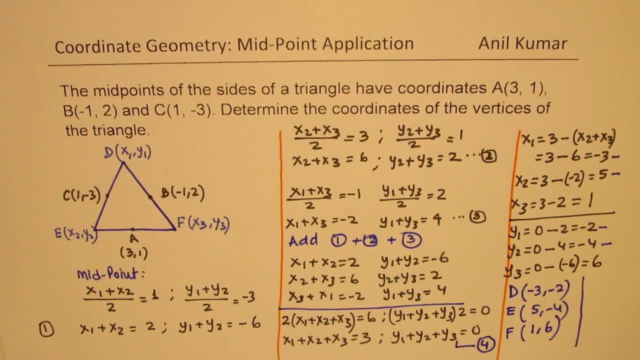 So these are simple steps to understand how to solve such a question. It's kind of easy to do now, right, once you understand the strategy, And that is In such cases. this is critical: Add them all to get the sum.